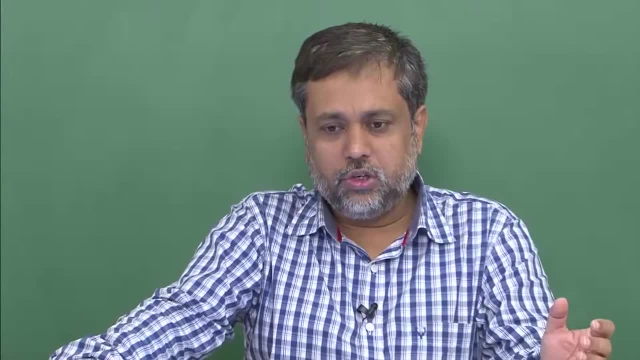 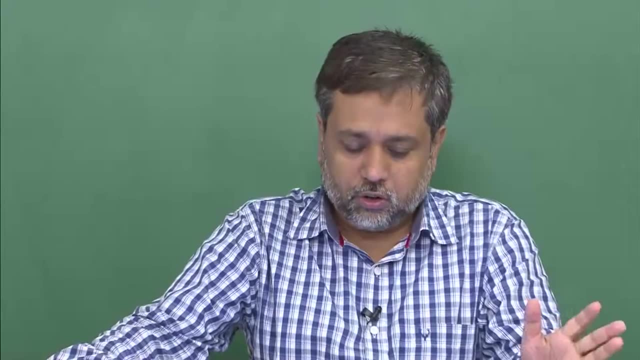 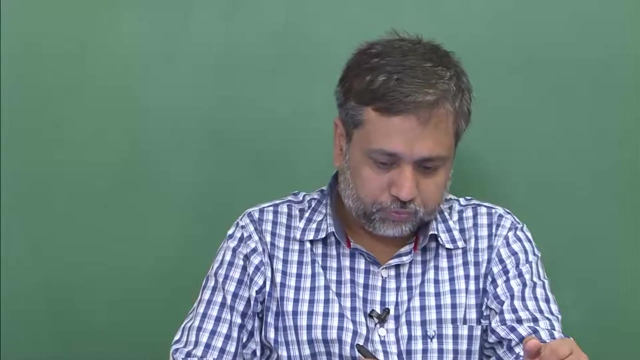 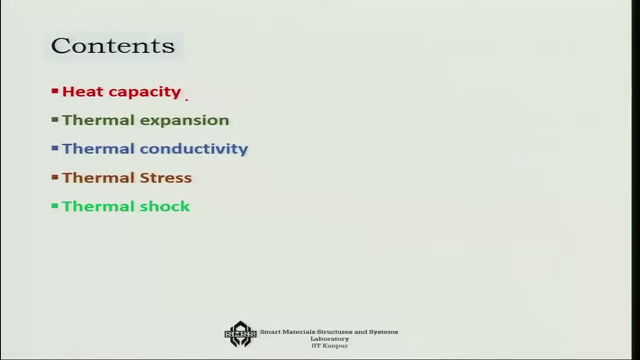 combustion engine. So hence there will be some heat which will be generated, and the heat is, you know, the temperature is to be kept within a particular level in order to safeguard many of your systems and hence the thermal properties become important. So, in this particular lecture, we will go through the heat capacity, the thermal expansion. 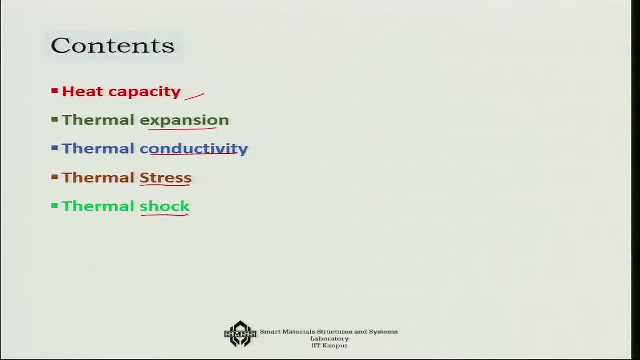 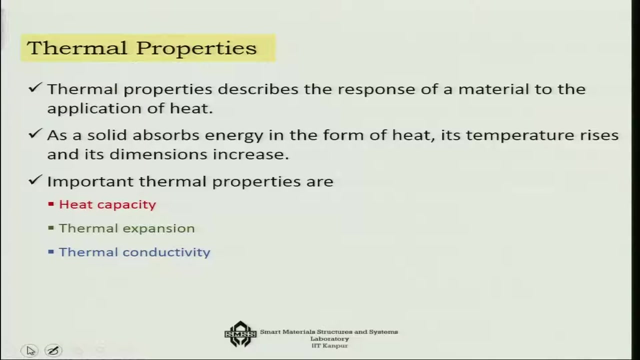 conductivity, thermal stress and thermal shock, the things which most commonly occur in most of the materials for engineering applications. Now, overall, the thermal properties describe the response of a material to the application of heat. As a solid absorbs energy in the form of heat. we know that its temperature. 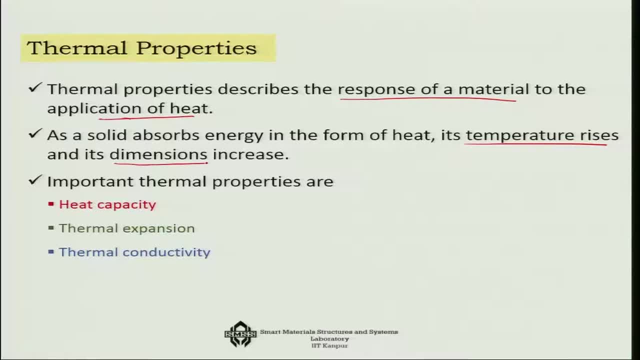 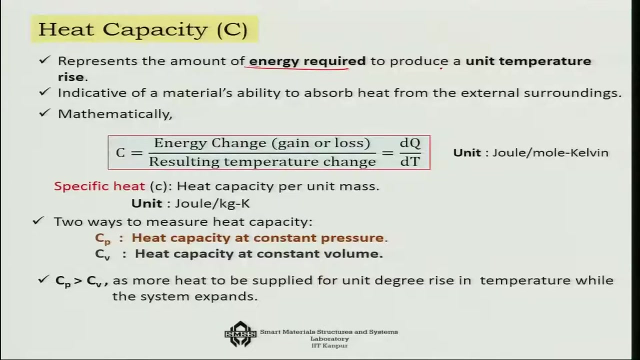 rises and its dimensions change. The important thermal property related to these are the heat capacity, the amount of heat that it is able to absorb per unit volume, thermal expansion and thermal conductivity. So heat capacity represents the amount of energy required to produce the unit temperature rise. Now this is indicated. 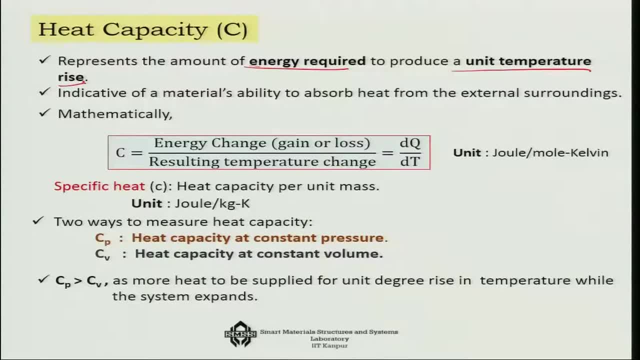 indicative of a materials ability to absorb heat from external surroundings, Because from the same unit, temperature increase. if you can absorb more energy, that means you have a higher heat capacity, and that is sometimes good, because you can actually, you know, in a small change of temperature by changing these or creating a small change of temperature. 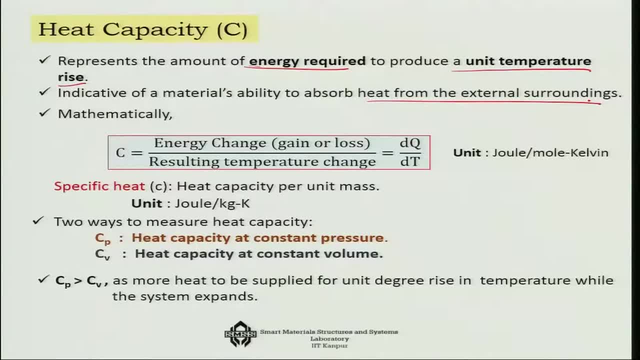 you can actually absorb much more energy inside the system. So mathematically this heat capacity C is defined as energy change. that is gain or loss. that is d cube over the resulting temperature change, dt. So its unit is joule per mole k. 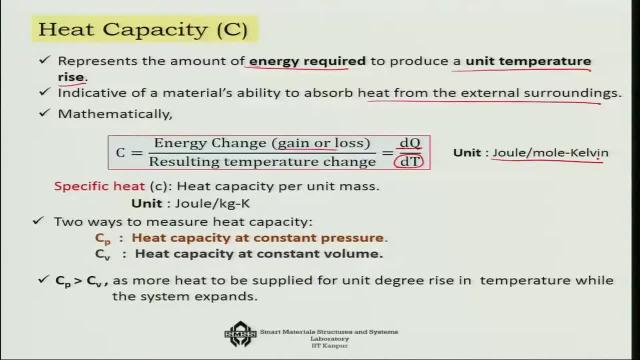 Now, along with this, there is a specific heat, which is heat capacity per unit mass, and its unit is joule per kg kelvin. There are two ways to measure the heat capacity. One is the heat capacity at constant pressure, Cp, and another is heat capacity at constant 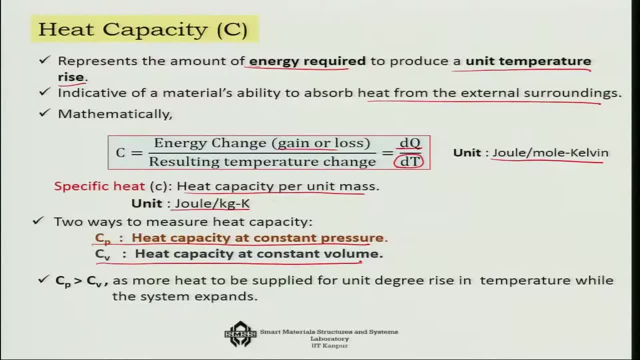 volume: Cp. Cp is greater, Cp is greater than Cv as more heat to be supplied for unit degree rise in temperature while system expands. So these are some of the basic things that are required in comparison, you know, in relation to the heat capacity of a system. 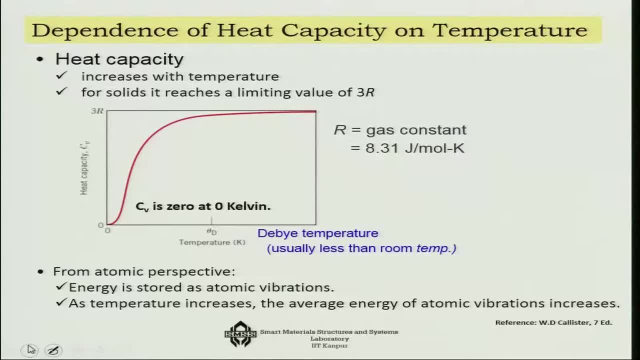 Now how the heat capacity changes with respect to temperature. First point is that it increases. First point is that it increases. First point is that it increases with temperature and for solids, however, it reaches a limiting value of 3R, where R is the gas constant: 8.31 joule per mole k. 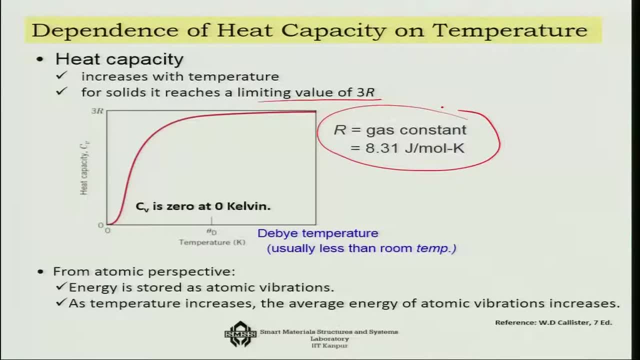 Now, the way it behaves is that, as the temperature is, in you know, gradually increased, there will be actually, you know, the atomic vibrations that will take place, So the temperature will increase. Now, with respect to the increase of temperature, the average energy of atomic vibration will. 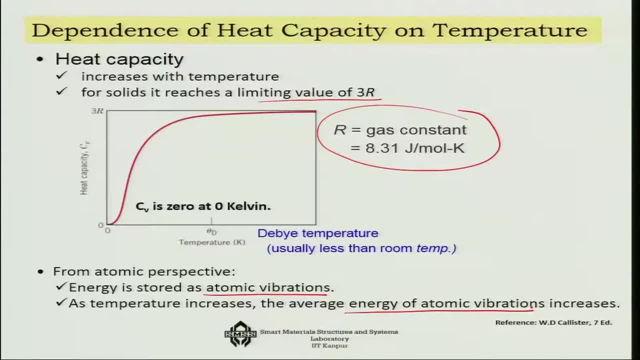 increase. However, atoms are restricted within a particular- you know- region. So hence you know there is a maximum level because of up to which it can actually exhibit this. you know energy increase Because you know there is a maximum energy, So it will increase because beyond that, the bond of strength will not allow it to go here. 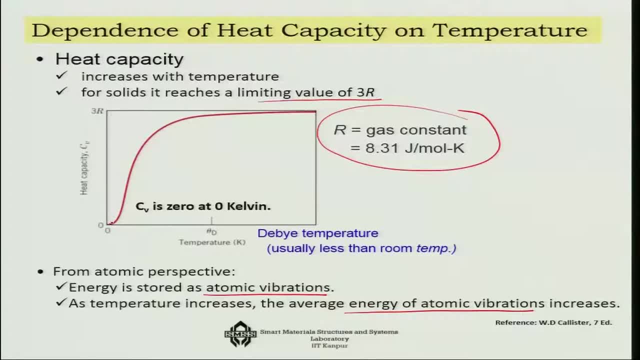 and there and, as a result, what you will see is that initially there is a sharp jump because the atoms are getting excited more and more, but in as you are reaching the 3R value- that is the maximum that is permitted- so it is coming down to a saturation. 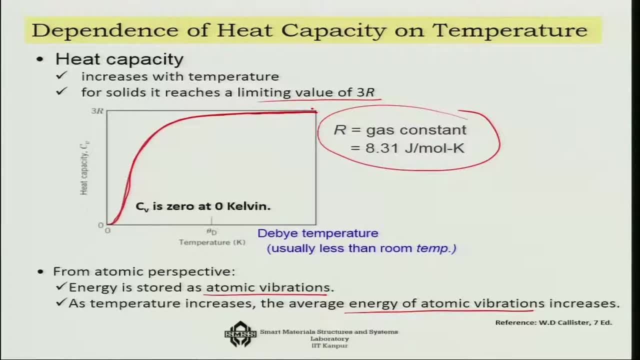 So that is how you know this particular thing happens. So what happens in the case of any material and there is a temperature which is called the Debye temperature and which is usually less than the room temperature, in which you will see that this saturation is happening to the system, 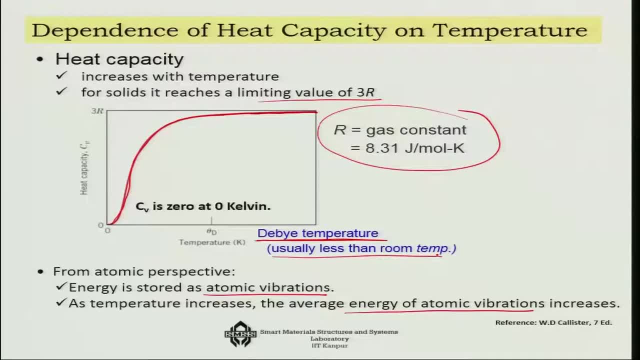 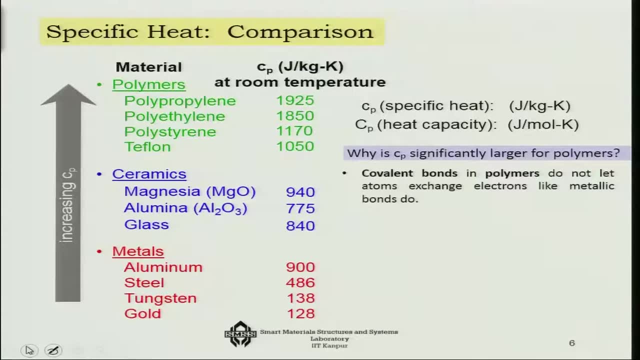 And various materials will show various Debye temperature. Now if I compare various materials with respect to the specific heat, That is, heat capacity per unit mass, then we have three groups of materials: polymers, ceramics and metals. What you will see very interestingly is that polymers have much higher heat capacity. 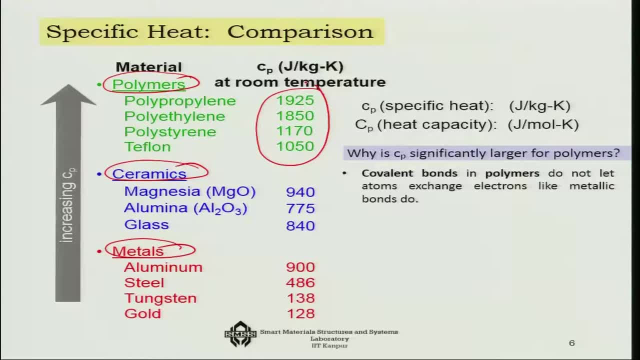 Polypropylene, polyethylene, polystyrene, teflon. they are much higher heat capacity. Next are the ceramics, and below that are actually the metals Among the metals. of course, some metals have higher heat capacity than the others. One important point is that there are covalent bonds in polymers that do not let the atoms 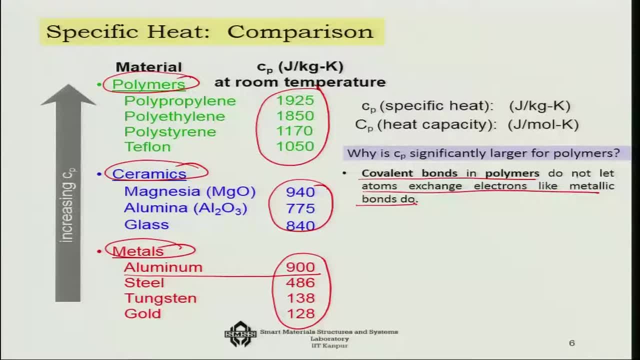 to exchange electrons, like the metallic bonds, because metals have free electrons and hence it can exchange the electron. So this also increases the temperature at a faster rate And as the heat capacity, you know, actually is inversely proportional to the increase of temperature, So the less there will be change of temperature, the better it is from the heat capacity point. 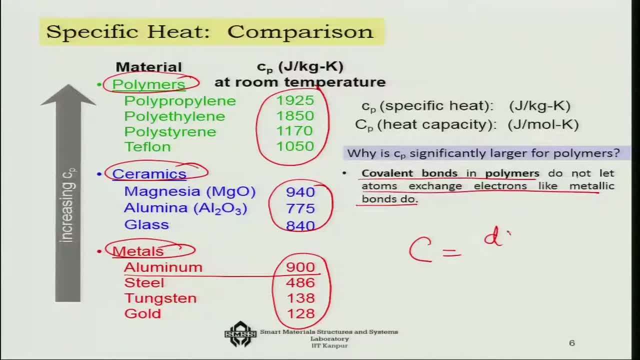 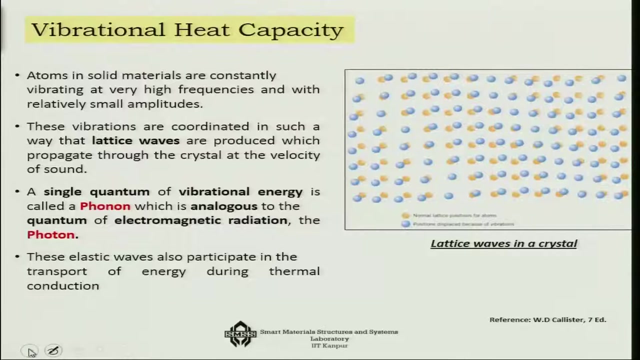 of view. I think you remember that C is d, cube dt, right. So for metals, because of the presence of free electrons, these dt is going to be more. as a result, Their heat capacity is less in comparison to the polymers. Now there is a way in which we actually describe this entire phenomena in solids. 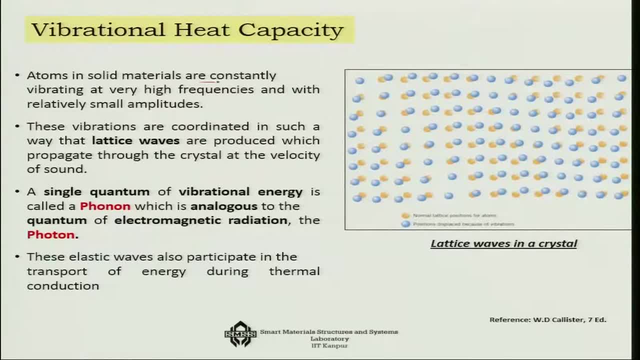 Atoms in solid materials are constantly vibrating at very high frequency and with relatively small amplitudes. These vibrations are coordinated in such a way That lattice waves are produced which propagate through the crystal at the velocity of sound, because this is not, you know, like your photons, or not like your, you know, electromagnetic waves. 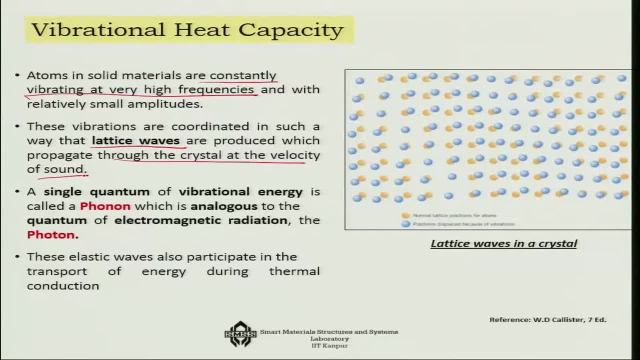 this is actually longitudinal wave, So it moves at the velocity of sound. A single quantum of vibrational energy is called a phonon here, which is analogous to the quantum of electromagnetic radiation, which is photon. Now, This elastic waves also participate in the transport of energy during the thermal conduction. 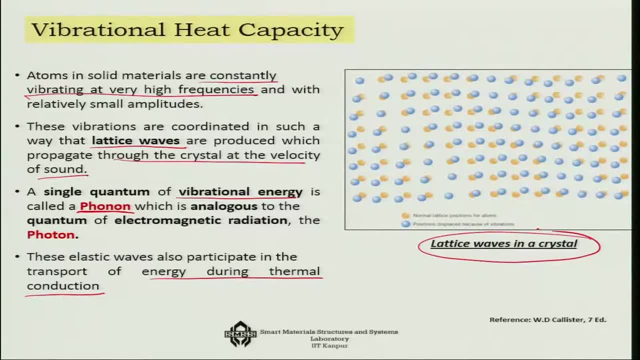 So here we have shown that there is a lattice wave that is generating in a crystal, and then you can see that the, you know, the phonons are actually getting displaced and thus, you know, with respect to this direction, you can see that the yellow lines are the normal lattice. 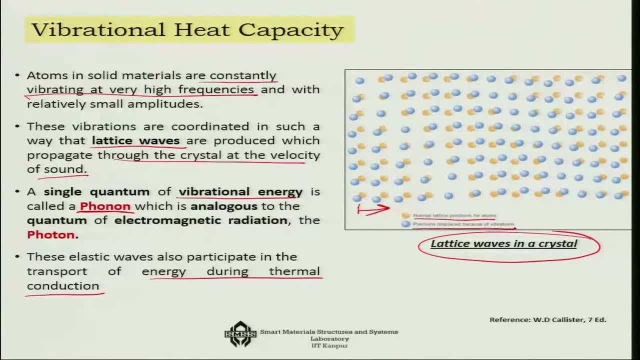 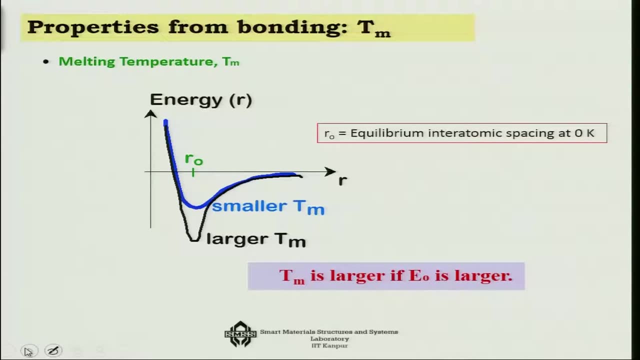 position. The blue lines are positions due to the vibration. So there is this continuous- you know this change that is happening and that wave is passing through the system. Now there are some important thermal properties which also can be explained from the point of view of atomic bonding. 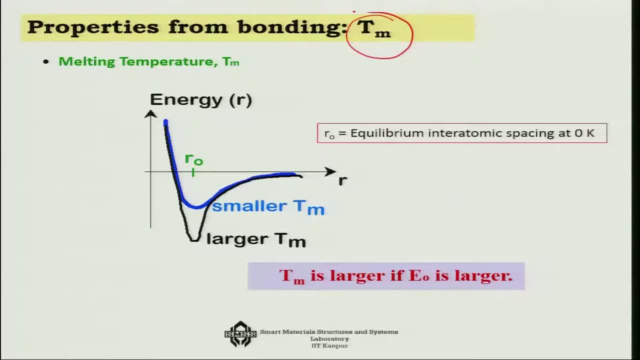 The most important of them being the melting temperature, Tm. Now, If you remember The ah, you know curve that we have drawn earlier for the bond energy, We have shown that there exists a particular- you know- position in the bond energy where the energy is the minimum and hence the bond becomes very, very stable. 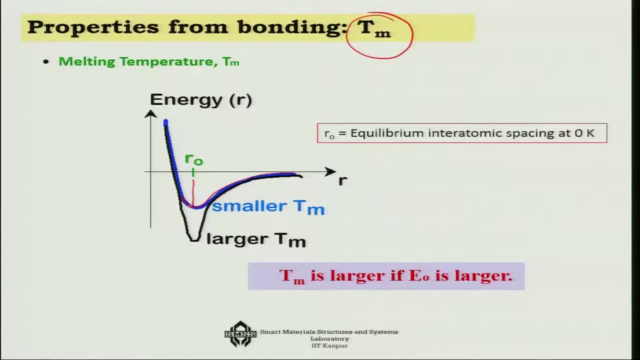 Now, what happens is that those materials which has actually ah larger, you know melting temperature, Now, If you remember The melting point, You will see invariably that they have modulus of elasticity which is also larger. and modulus of elasticity, if you remember, actually talks about the inter atomic. you know bonding. 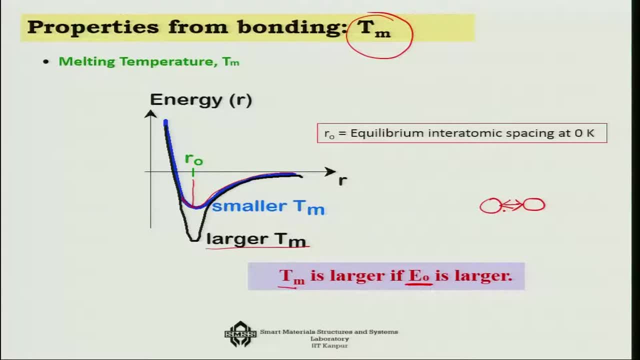 So that bonding force is actually much more okay in in the ah, you know in the materials, which has actually larger ah, you know the melting point. Or in other words, if the bonding force is more, then you need more energy to generate the flow system and hence Tm is larger for this type of a system. 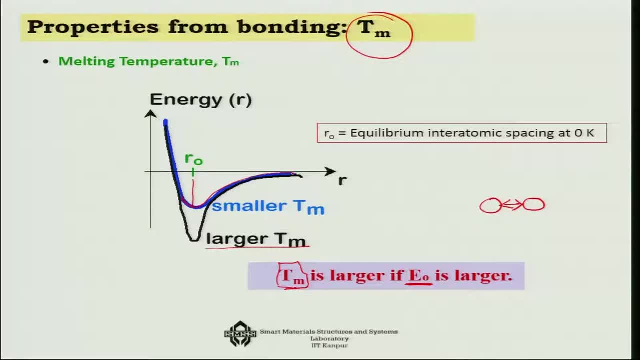 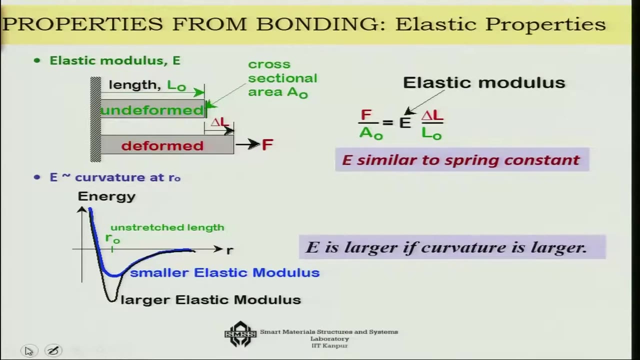 So for, ah you know, a typical energy curve for a material with larger Tm will show actually more ah, ah drop in the system in comparison to the material with this smaller Tm. Now, From the bonding point of view, the elastic property, ah you know, is very important and 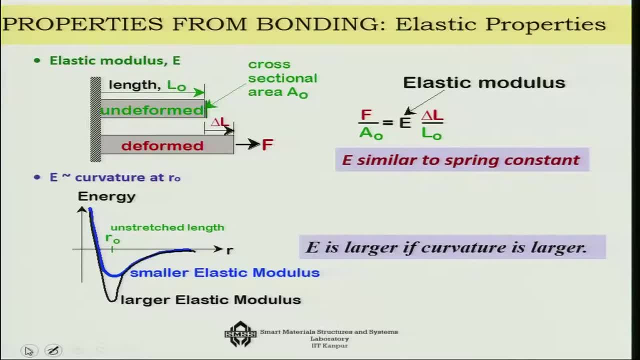 you can also see it in this way, that suppose you have considered a particular strip which is undeformed, of length L0, okay, and cross sectional area is A0. Now you are applying force F and then it is deformed, and then there is a change of length. 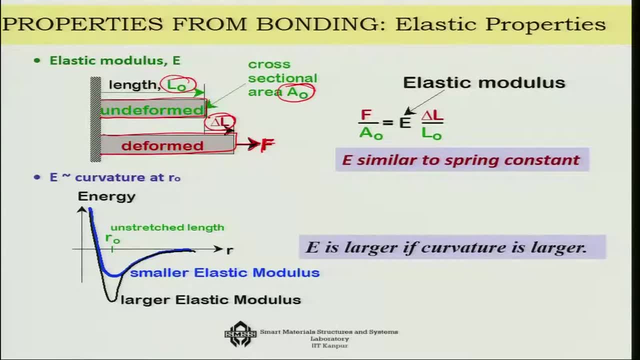 which is delta L. So what is the stress that is generated in the system that is F over A0, and why, how it is related to the strain that is E that is generalized. there is the Hooke's law: E times the length change, change of length over the original length, which is nothing but the epsilon. 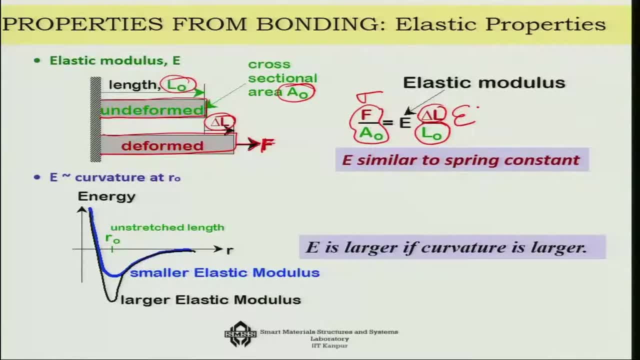 So sigma equals to E, epsilon. E is thus similar to A0.. Okay, That is the spring constant. And then if you look at that, you know E is the curvature at R0. then you can say that those materials which are having the larger elastic modulus at R0, they have a sharp curve. 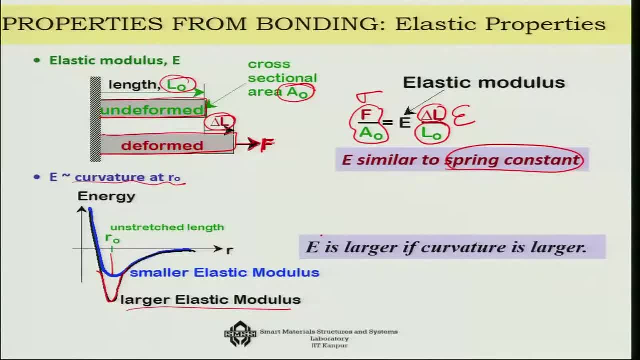 the curvature is higher. So modulus of elasticity, Okay, The modulus of elasticity is actually larger if the curvature is larger. On the other hand, modulus of elasticity is smaller, if you know, the curvature is small, as is shown in this particular case. So thus, from the curvature point of view, also by looking at the bond energy, you may say- 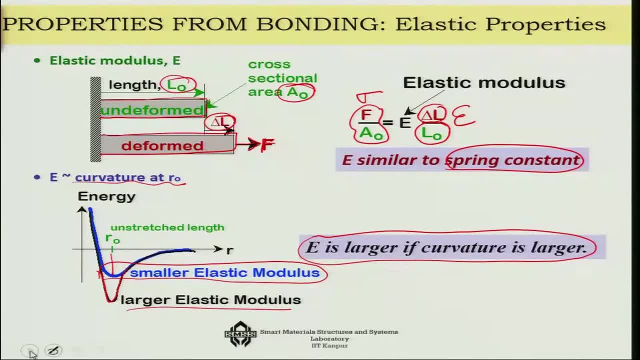 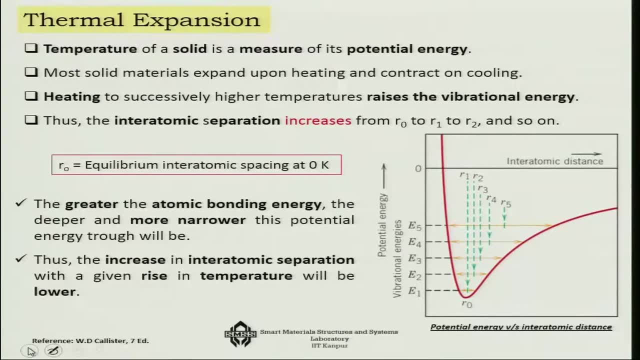 that, between the two material, which one is possessing Higher modulus of elasticity. Next we talk about thermal expansion and, as you know, that temperature of a solid is also measure of its potential energy in some sense. Now most solid materials expand upon heating and contract on cooling. 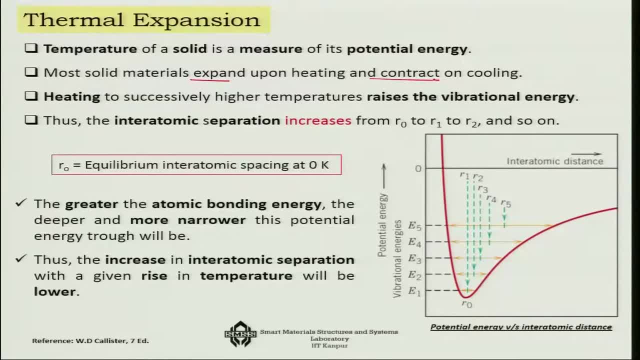 There are exceptions. we have seen, for example, shape memory alloy wires which actually, upon heating They will show sharp contraction due to the phase change. But normally solid materials will expand upon heating and contract on cooling. Heating to successively high temperatures raises the vibrational energy. 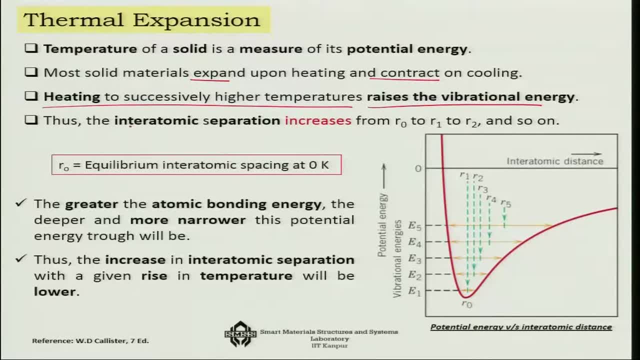 Thus, as the vibrational energy increases, the inter atomic separation increases. So from R0 you are going gradually to, you know, R1, R2, R3, R4, R5, up to a particular distance. So the greater the atomic bonding energy, the deeper and more narrower these potential energy. 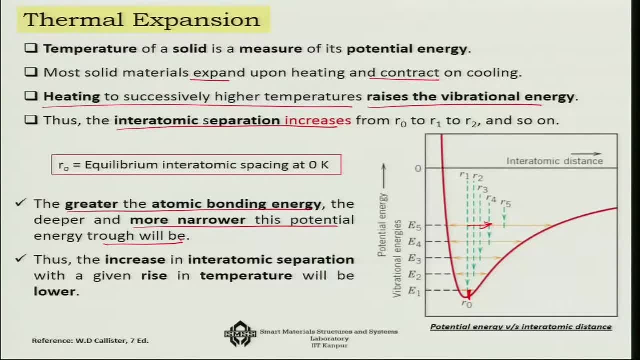 trap will be, And thus the increase in inter atomic separation with a given rise in temperature will be actually lower. Because we already told you that, in comparison to the ah, you know things with the smaller bond energy, these are actually sharper here. So the greater the atomic bonding energy, the deeper and more narrow these potential energy. 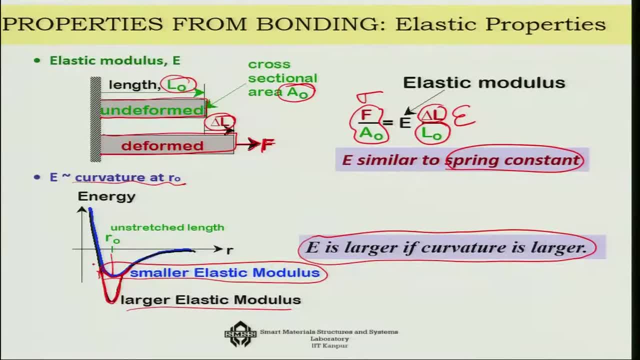 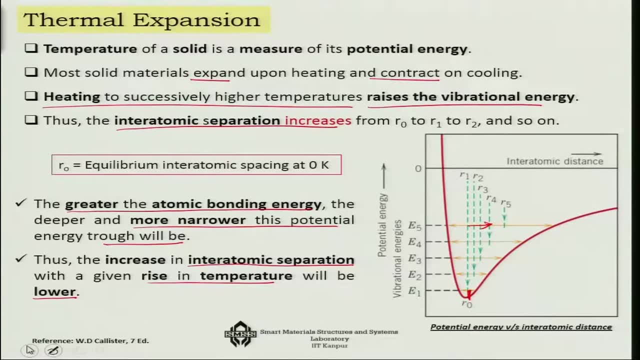 traps will be, As you can see, in comparison to the one with a smaller bond energy. So, since it is sharper, so the increase in inter atomic separation with a given rise in temperature will be- ah, you know, ah, lower in this particular case. So as a result, ah you know, the thermal expansion coefficient will be actually lower. 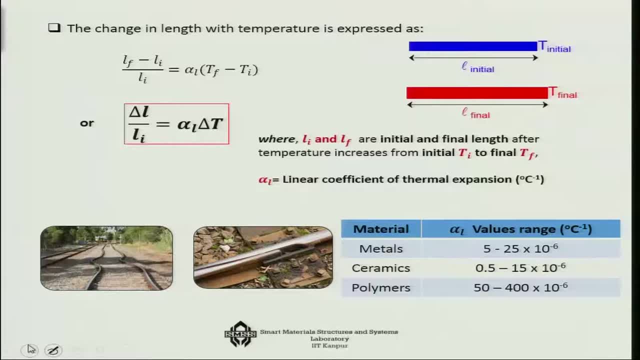 If we try to ah see that in terms of the thermal expansion coefficient definition first, which says that is the relationship between, you know, change of length over original length and the change of temperature. So essentially alpha, you can write it as alpha is delta L over L over delta T. So when L i 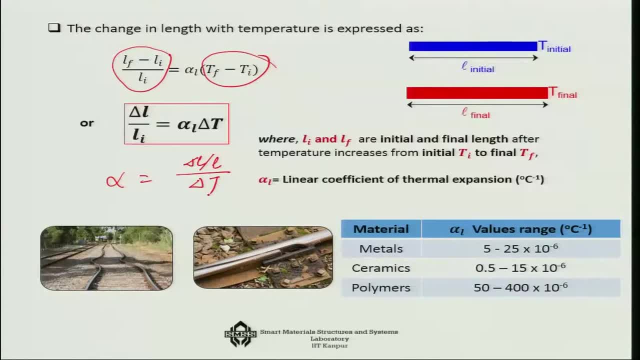 and L f are the initial and final length after temperature increases, from initial T i to final T f, and alpha is the linear coefficient of thermal expansion. Following this definition, metals have a thermal expansion coefficient which is like 5 to 25 into 10 to the power minus 6 per degree centigrade. 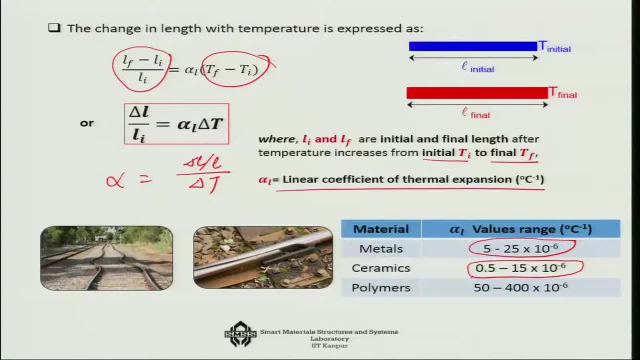 Ceramics: 0.5 to 15, lower than 0.5.. Okay, More than the metal And polymers. it is very, very high, 50 to 400, significantly higher than the metals, And you can see it here that, with respect to a unit change of temperature, you would. 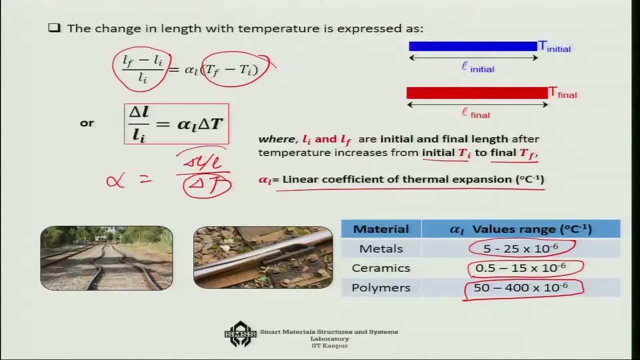 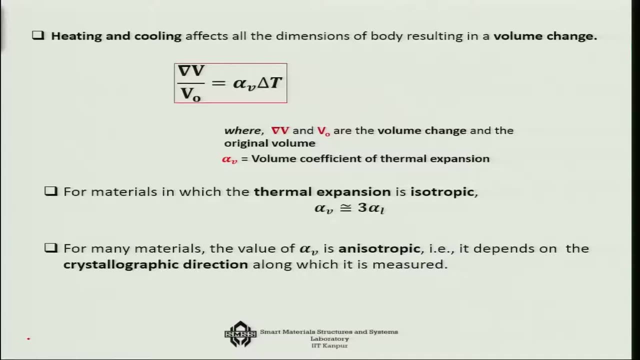 actually see in polymers more change in length in comparison to the metals, And that is because the polymers offer- because of their less bond energy, they are actually offering much more change. Now the heating and cooling affects not only in one dimension, but it affects the entire. 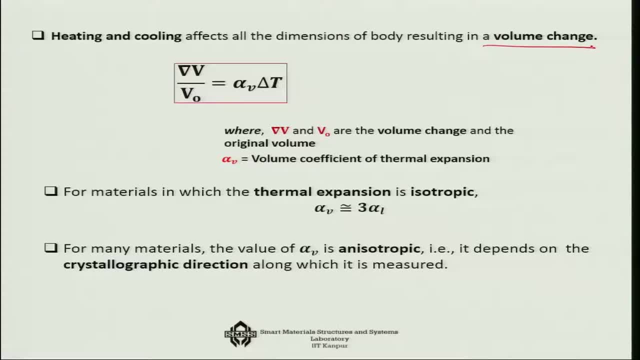 you know all the three dimensions, since the volume change as well. So, similar to alpha in one direction, you can also define a alpha v which is like delta v over v0.. So alpha v, So alpha v, is your delta v over v over delta t. 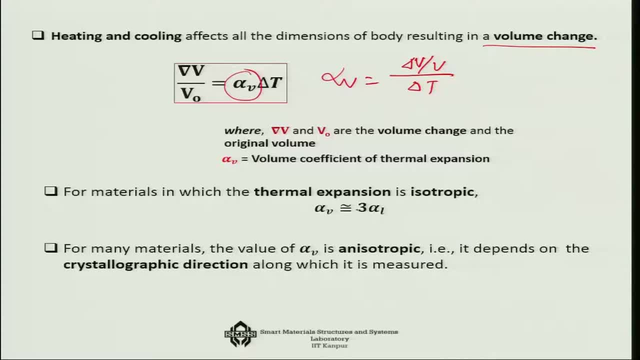 So alpha v in general, you know, for isotropic thermal expansion it is about three times of alpha 1.. But some cases, some materials, alpha v is an isotropic. that means the material expands at a different rate in different directions, for example crystallographic directions or 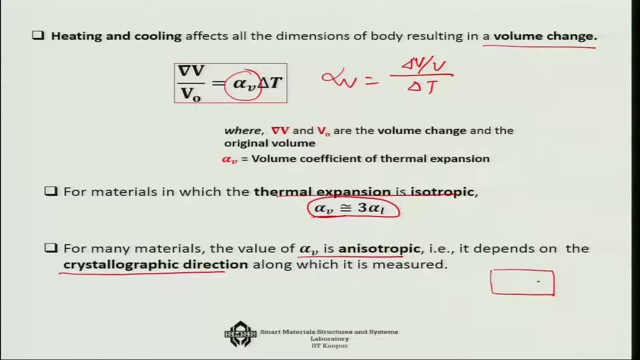 for example. So we consider, you know a fiber reinforced composite, then along the direction of the fiber it has one coefficient and you know, across the direction. so in these two directions it has two different thermal expansion coefficient. So these are an isotropic cases. Otherwise, for isotropic cases, alpha v is approximately three times the alpha l. 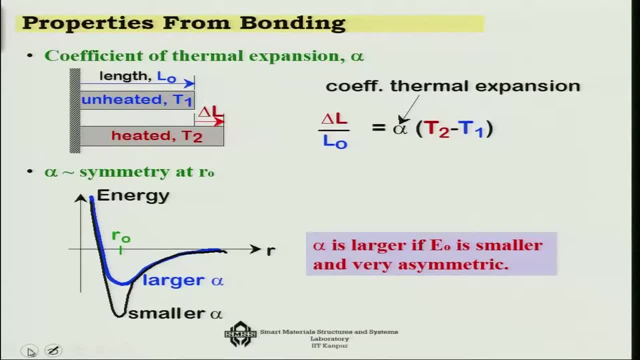 Again, we can explain the thermal expansion coefficient. So what is this? z i From onerandy 90. We can explain the thermal expansion coefficient from the properties of bonding. As you know, we have earlier shown you that the same expansion of the unheated and the 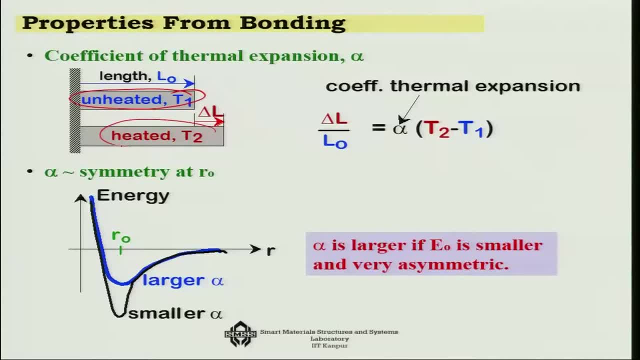 heated beam. if you consider and suppose the change in length is delta L, So for the same change in temperature, what you will see is that in some material this delta L is will be much more, and alpha is actually your delta L over L0 over delta T. 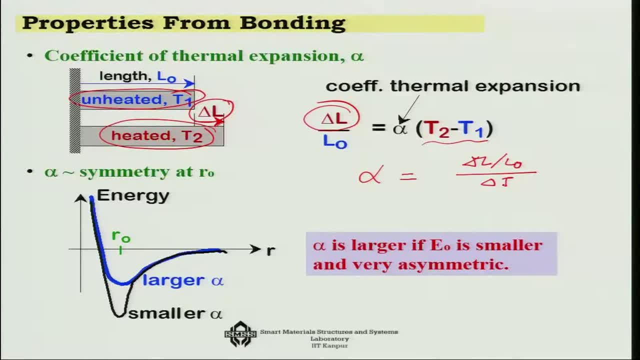 So, if you know, delta L over L0 increases more in comparison to delta T, Okay, Okay, Okay, Okay, Okay, then you are going to get a higher value of alpha. So alpha is larger if E 0 is smaller. 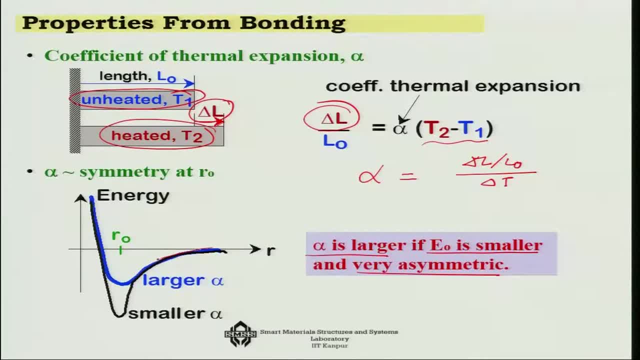 and very asymmetric. Why? because for a softer material, for the same change in temperature, you may see that it allows more change in the inter atomic distance because the bond energy is less in comparison to the- you know, the other material. So, as a result, alpha, 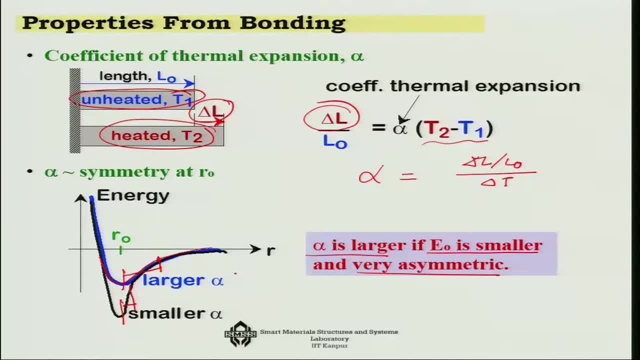 is larger and if E is smaller because for this material E is smaller, So E is smaller and in comparison to this particular material. So in this case E is higher. Higher the E, narrower will be this curve And smaller will be alpha. Lower the E, larger will be this curve and higher will. 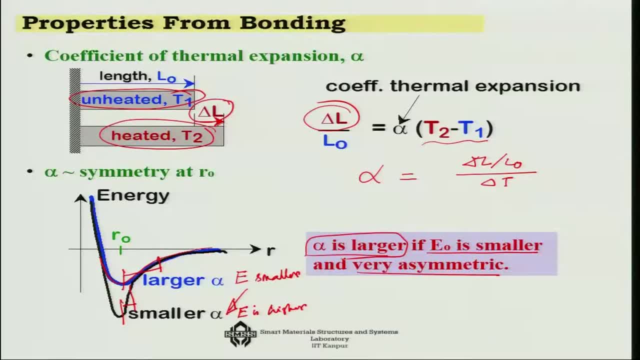 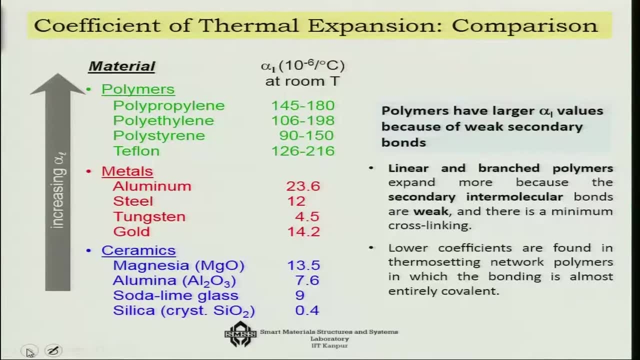 be the value of the alpha. That is the point we have to keep in our mind. Next, if I compare the thermal expansion coefficient, we will see that this is indeed getting reflected. You get a large thermal expansion coefficient for all the polymers Metals it come down. 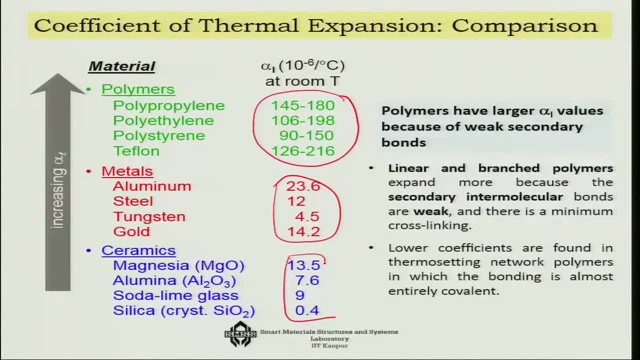 and then it goes down. So this is the thermal expansion coefficient for all the polymers, Ceramics. it also comes down further. Now polymers have larger alpha L values because of the weak secondary bonds. It allows it to move further, In fact linear and branched. 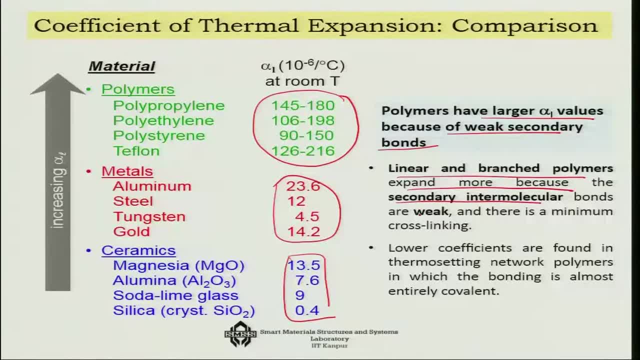 polymers expand more because the secondary intermolecular bonds are very weak and there is minimum cross linking. Lower coefficients are found in thermosetting network polymers, in which the bonding is almost entirely coherent. Now, in comparison to the polymers, bond energy is much higher in metals and ceramics and 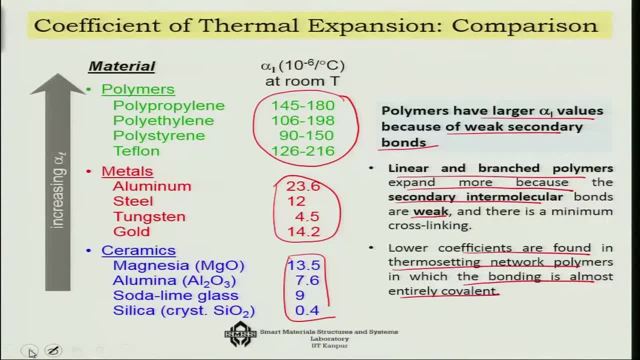 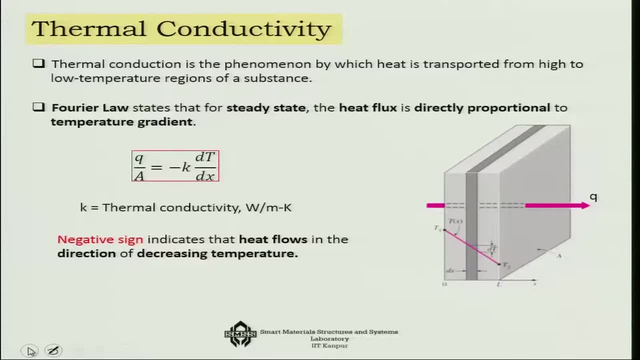 as a result, alpha is much, much smaller in these cases. Next is the thermal conductivity. Thermal conduction is the phenomenon by which heat is transported from high to low temperature regions of a substance, And there is a particular law which is known as Fourier law. 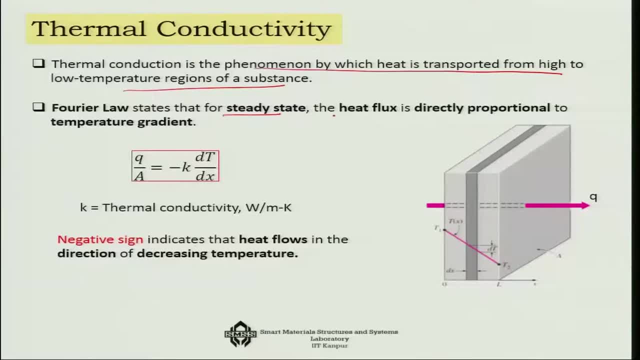 Fourier's law that states that for steady state the heat flux is directly proportional to the temperature gradient. So the relationship is something like this: that Q over A is minus k, dT over dx And the negative sign here indicates that heat flows in the direction. 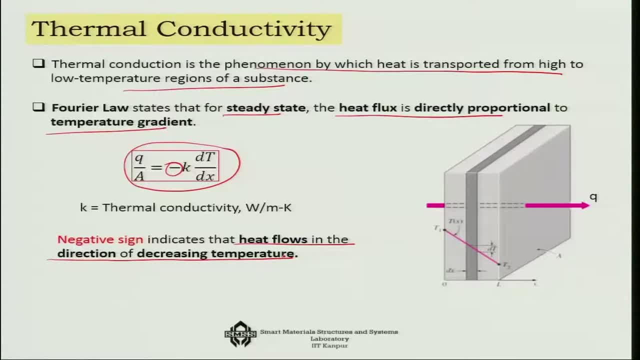 of decreasing temperature. So from high temperature to the low temperature, towards the low temperature, the heat is flowing. So that is the Fourier's law, which actually brings this thermal conductivity k into picture for us, which is measured in terms of many units are there, but one common is watt per meter Kelvin. 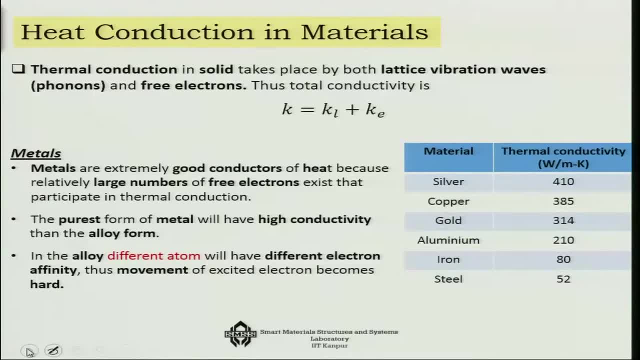 Now, if you look at it how the heat conduction takes place in materials, Then you will see that there are two ways in which it happens. One is thermal conductivity and the other is thermal conductivity. Now, if you look at it how the heat conduction takes place, 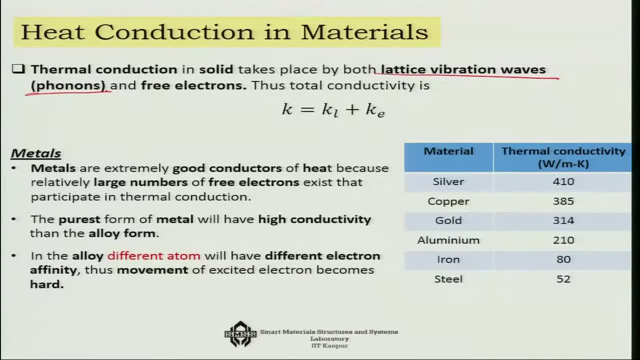 is through the lattice vibration wave, So to say through the phonons, and the other one is through the free electrons. So thus the total conductivity is partly due to phonons and partly due to the free electrons. Now, metals are extremely good conductor of heat. Why? Because it has relatively large. 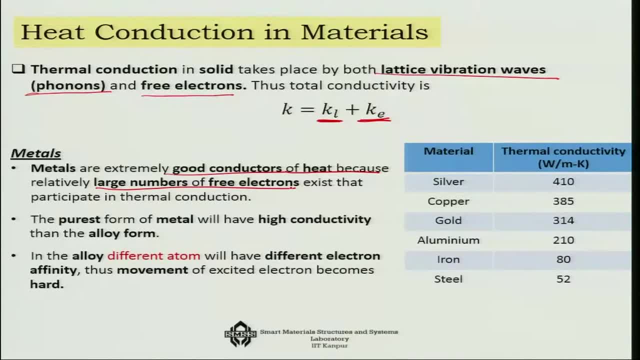 number of free electrons, So that takes care of the conduction. The purest form of metal also will have higher conductivity, So it will have higher conductivity. So it will have higher conductivity in comparison to the alloys, Like if you compare iron, which 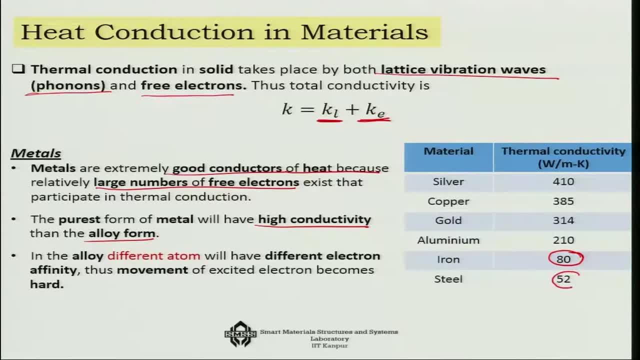 has thermal conductivity of 80, in comparison to that steel has 52 only, Because whenever you have alloying then you have less availability of free electrons and as a result you know the heat conduction comes down. If the alloy in the alloy, different atom will have different 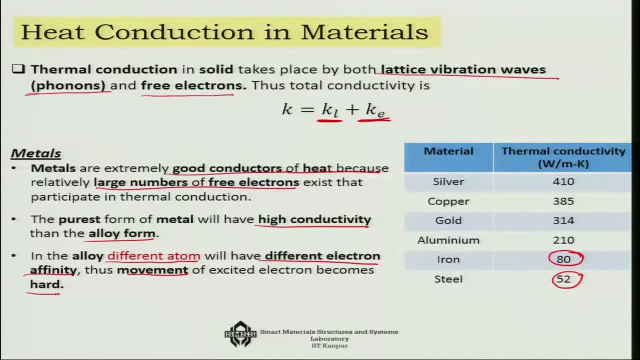 electron affinity. thus the movement of excited electron becomes hard. So that is why the electron becomes hard. in this case- And there are some materials where the phonon is more than the free electrons, For example ceramic materials- The free electron availability is very, very less, because mostly it is electrovalent. 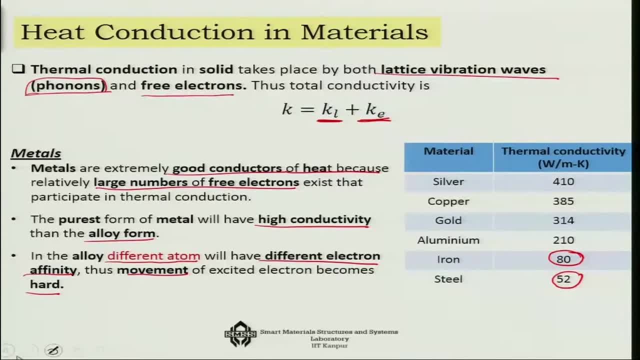 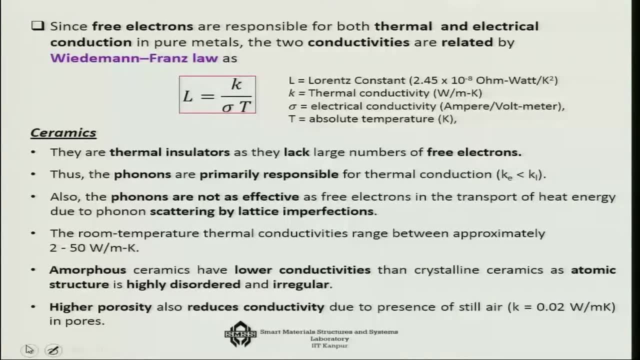 bonding. So there the phonons actually, you know, dominate in terms of heat conduction. So, in the case of pure metals, the two conductivity properties are related by a law which is called Weidmann-Frainz law, where the thermal conductivity and electrical conductivity are related together, and this is defined by a. 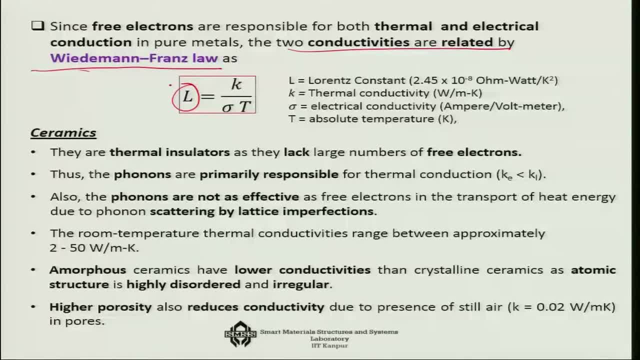 Lorentz constant L, where K is our thermal conductivity, sigma is the electrical conductivity and T is the absolute temperature. Now in ceramics they are thermal insulators as they lack large number of free electrons, So the thermal conductivity is very high, So the 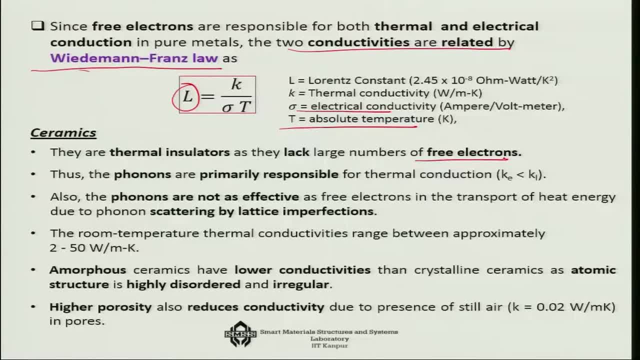 thermal conductivity is very low. So we can say that the thermal conductivity is very low, But the thermal conductivity is very high because there is a large number of free electrons. So free electron base transfer does not take place, Only the phonons are. 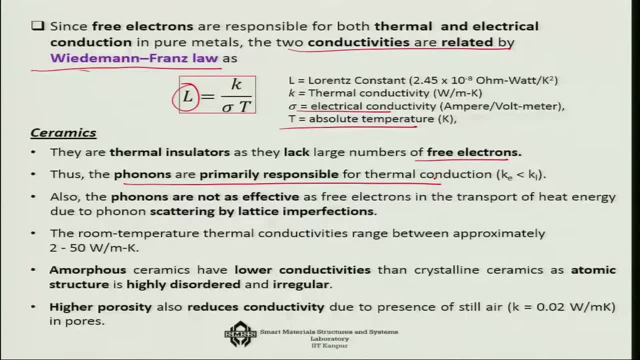 primarily responsible for the thermal conduction. Also, the phonons are not as effective as free electrons in the transport of heat energy due to the phonons scattering by the lattice imperfections. So as a result, the overall thermal conductivity comes down for the same. 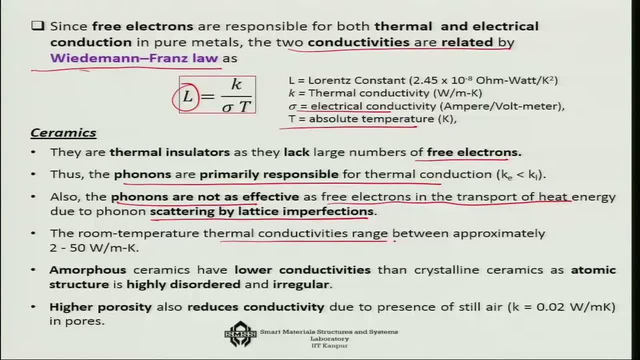 ceramics. The room temperature thermal conductivity is range in ceramics between 2 to 50 watt per meter Kelvin. Now, amorphous ceramics have even lower conductivities in comparison to the crystallines one, because crystalline ones have a regular, you know ordered structure. 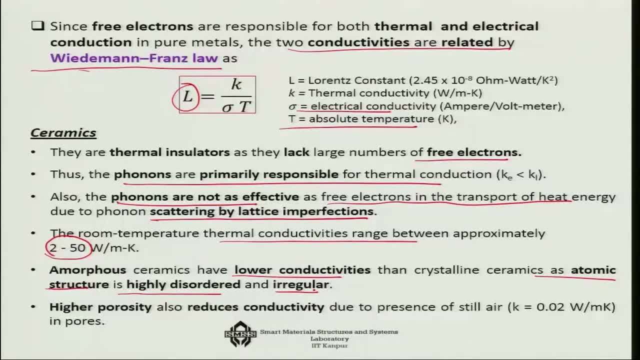 whereas amorphous are highly disordered and irregular. So the phonon phonon excitation is much lower. the damping is more. Higher porosity also because in ceramics they have high porosity. that also reduces the conductivity due to the presence of steel. air, because steel 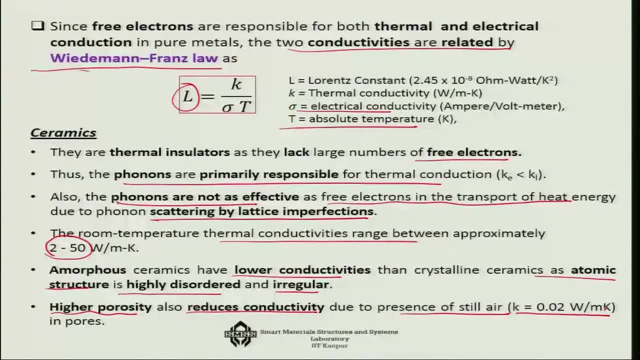 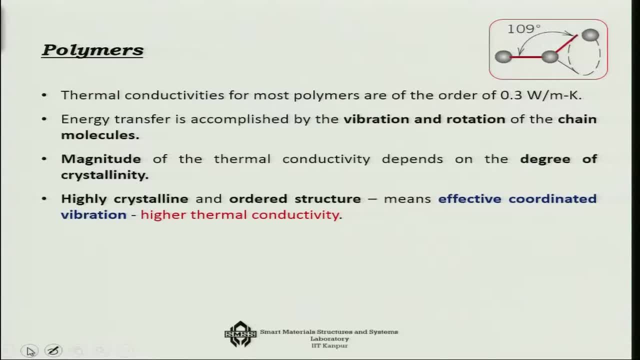 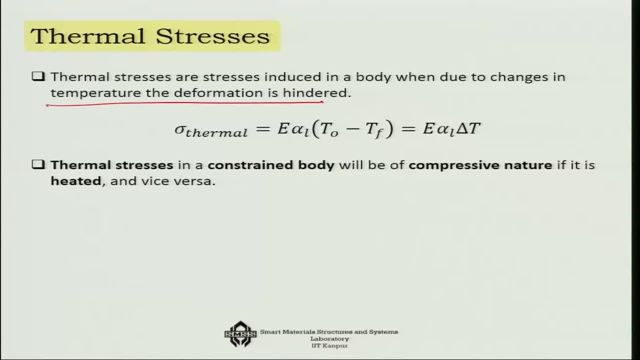 80., 81., 82., 82., 83., 82., 83., 84., 83., 84., 84., 85., 85., 86., 87., 86., 86.. 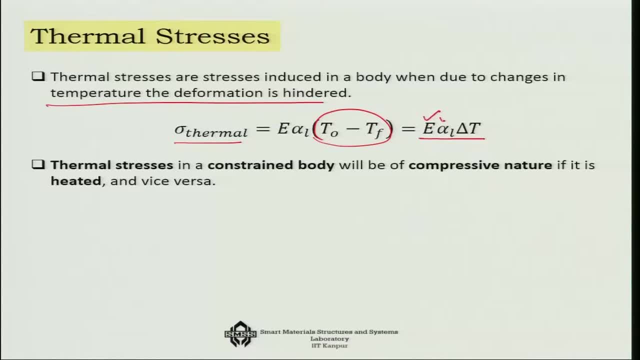 87., 87., 86., 87., 86., 87., 86., 87., 88., 88., 88., 89., 90., 91., 92., 92., 93.. 93., 94., 92., 93., 94., 95., 97., 97., 98., 99., 100., 92., 93., 0., 00., 99., 1..